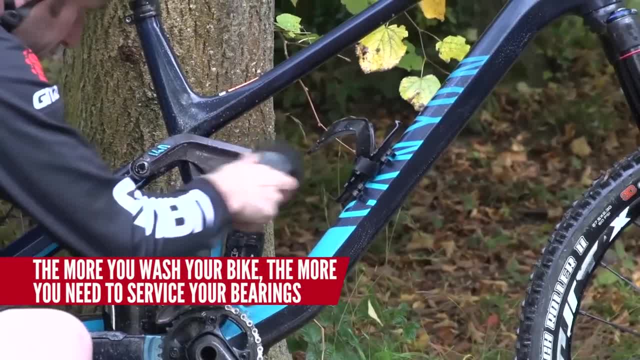 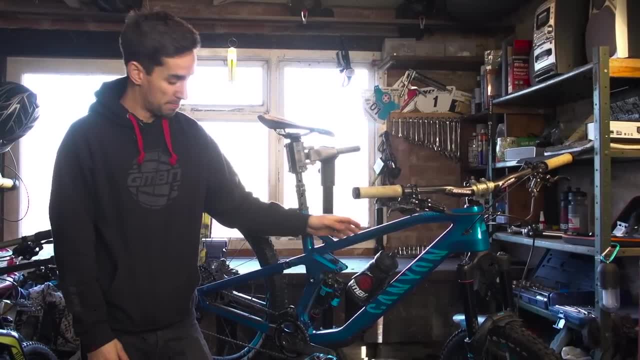 and actually the more you wash your bike in general, the more you'll have to keep those bearings nice and greased. So how do you service your bearings? Well, actually, some of them you can't. Most bottom brackets are sealed units, so when they start to get rough and worn out, 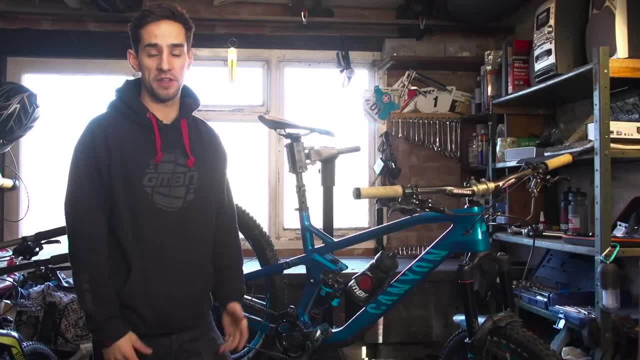 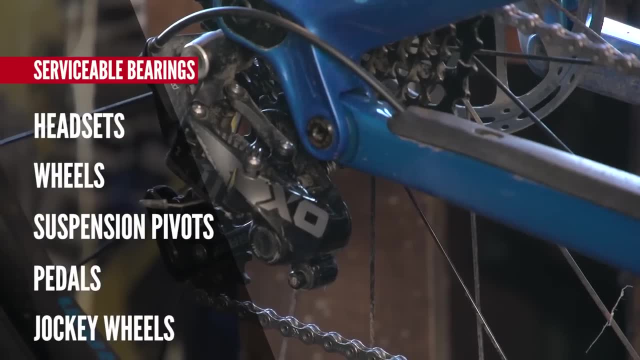 it's just time to replace that bottom bracket. But there's plenty on the bike that you can look after: Headsets, wheel bearings, suspension, pivot bearings, pedal bearings and jockey wheel bearings. You might find your bike has a few different types. 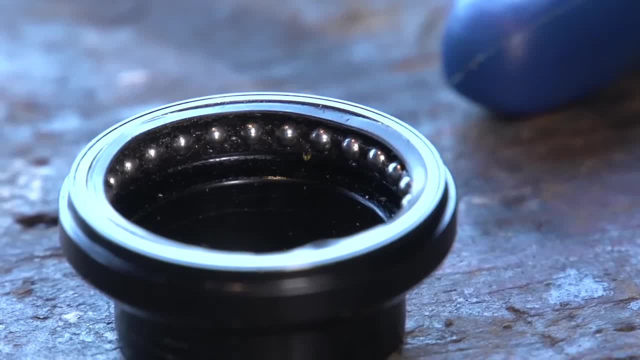 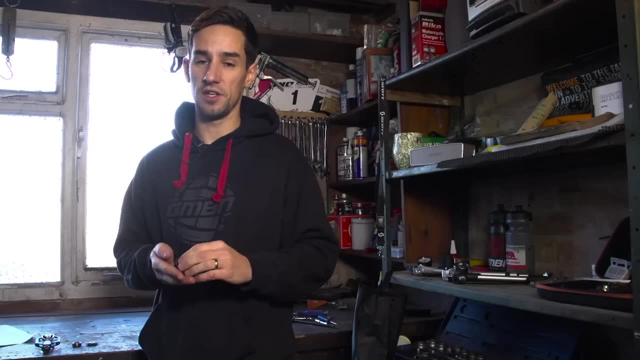 of bearing sealed or loose open bearings. Actually, the better quality of the components, the more often you'll find they have sealed bearings and, by their nature, less dirt gets into those bearings. The exception to this rule is actually Shimano hubs. 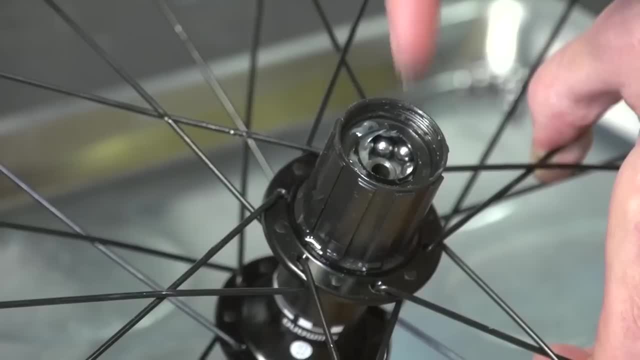 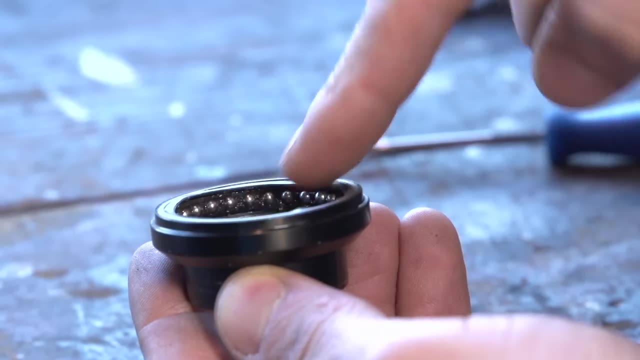 that use open cone and cup system because they believe they have less friction in those bearings. You can see this headset has loose bearings in there. You can see the ball bearings are in a race that just rolls around against this tapered surface and that's what helps your headset spin. 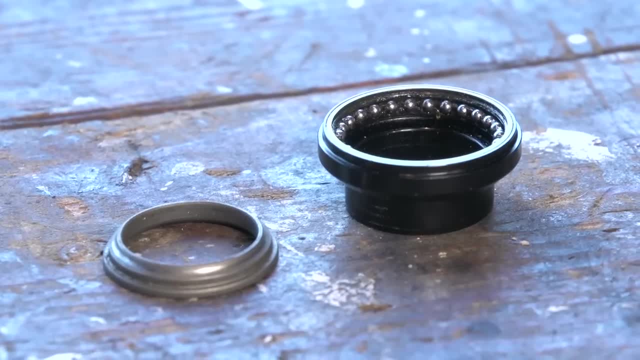 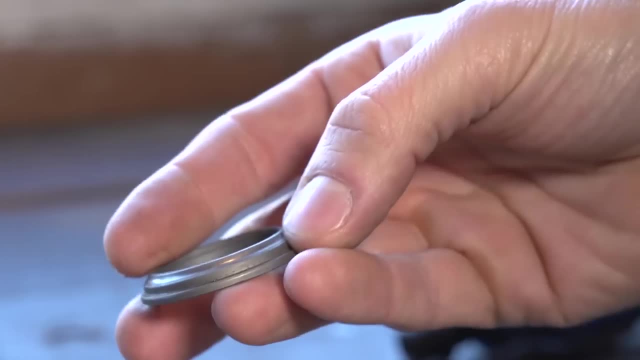 So it's really important that tapered surface is nice and clean and there aren't any sort of pits in there. Get those. if you'll get your headset really wet and leave it to rust in one spot, You might find the bearings just make a little hole in there. 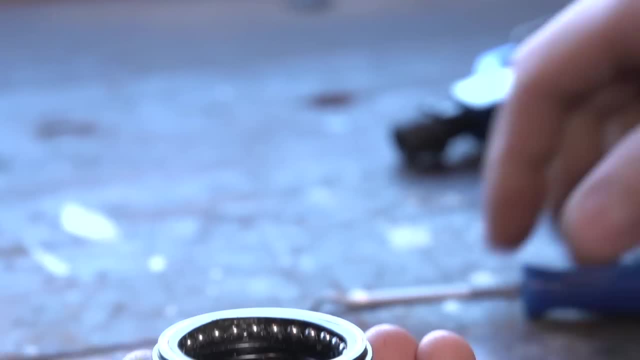 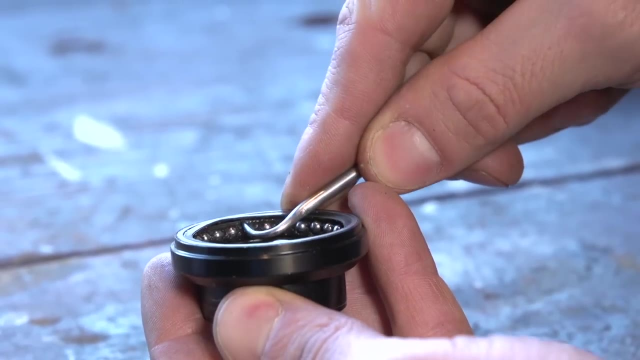 and it's never gonna spin very nice if you do that. So it's really important to keep them clean and rust-free. So what you can do generally is: I'll have this little plastic sort of seal on there. Just, really carefully, just pick that off. 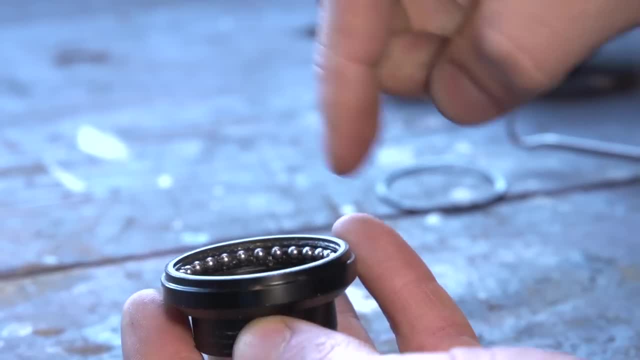 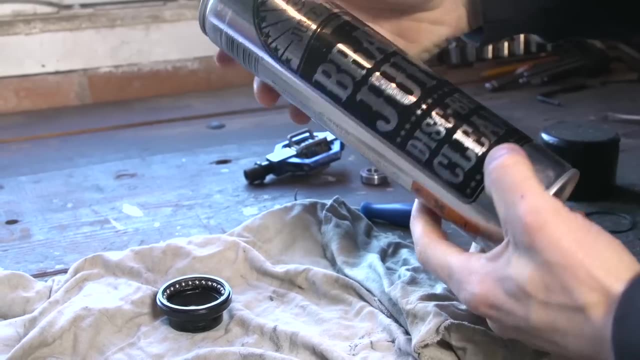 like trying to deform it, and now I can get into those ball bearings and give them a really good clean-out. So I've got myself a rag and I'm gonna use some solvent. I like to use disc brake cleaner, but any sort of degreaser will work. 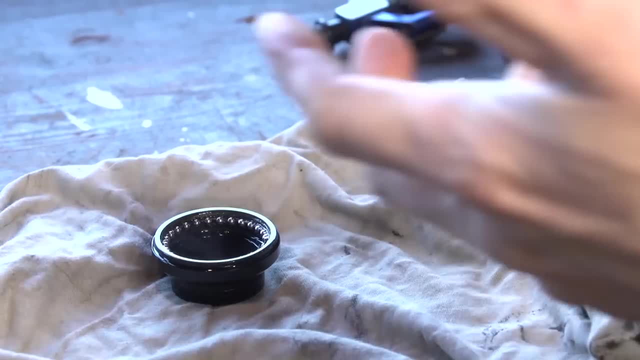 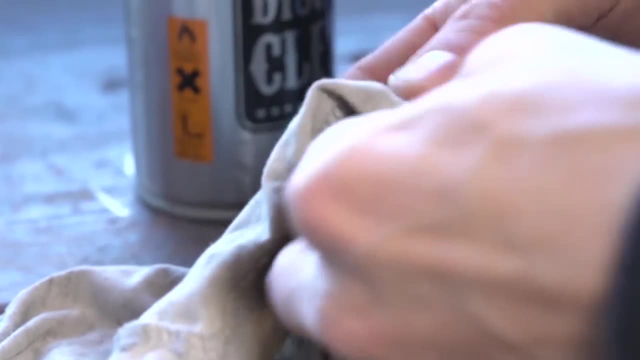 and it's just gonna get in there and get rid of any of the old grease that's holding on to that dirt and grime. So give it a real good wash out. Use your rag to get rid of any of that old grime. 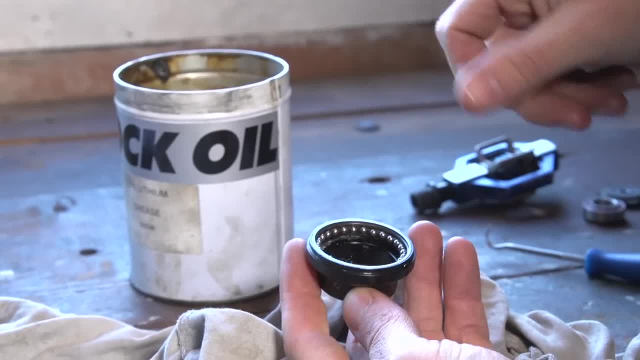 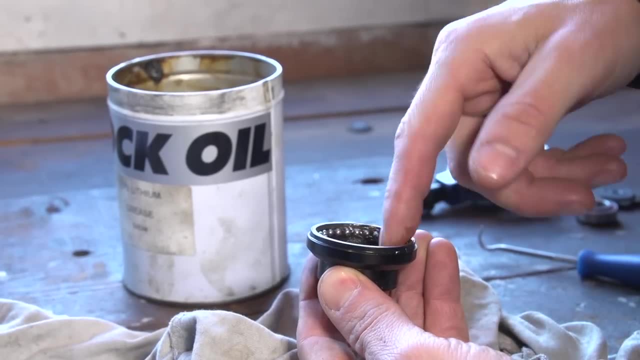 and you can feel it spinning nice and free now. So with those ball bearings dry, I'm gonna get in there and just re-grease it with some fresh grease. Don't go too mental, but just make sure they're nice and covered. spin them around slightly. 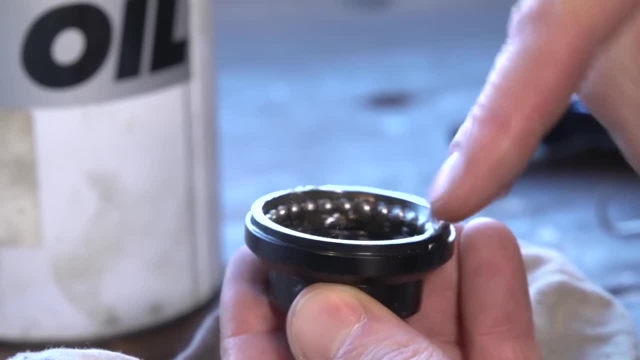 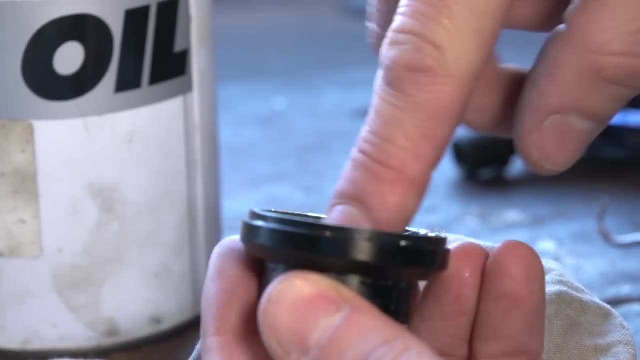 And the truth is you can get all sorts of things and lots of different types of grease, but it doesn't really matter As long as you're doing it nice and regularly. I like to use a fairly lightish. I don't go too thick with the grease. 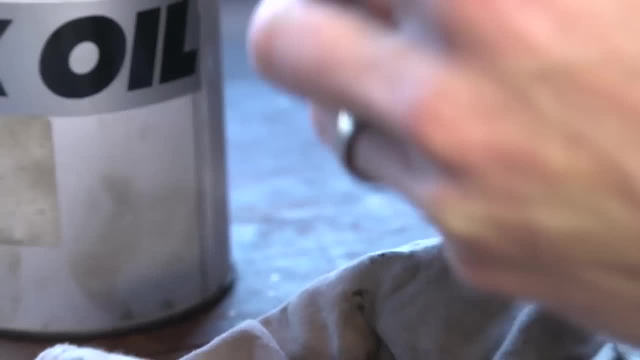 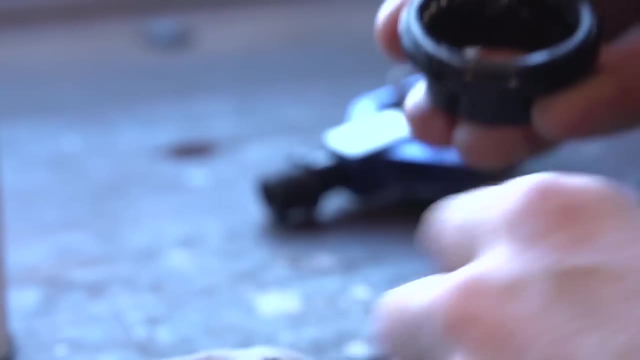 but make sure they're nice and greased. And same with the tapered sort of race that goes into that bearing. Just put a little bit of grease on that, Put your seal back on. Make sure your little tapered race is ready to roll. 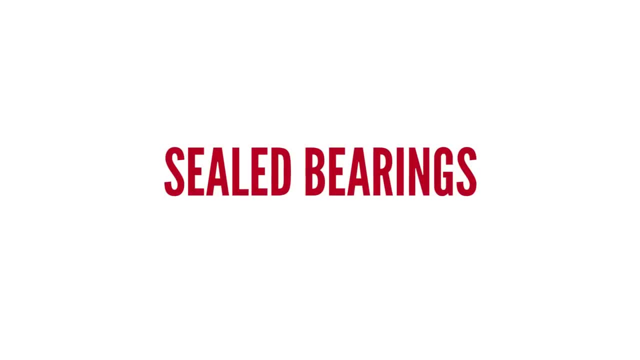 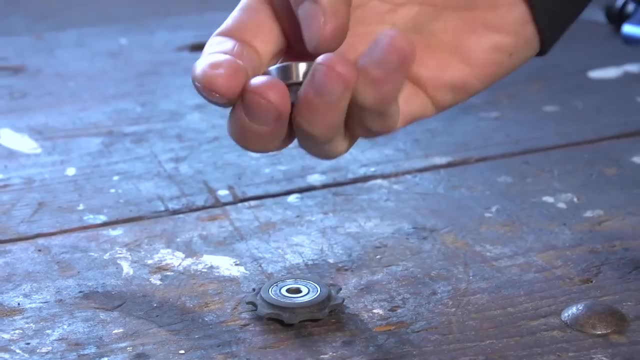 And there's your headset, nice and greased up and should spin freely again for a while. These are seal bearings You'll often find on your suspension linkage, your jockey wheels and also sometimes in your headset. You can see they're out of race. 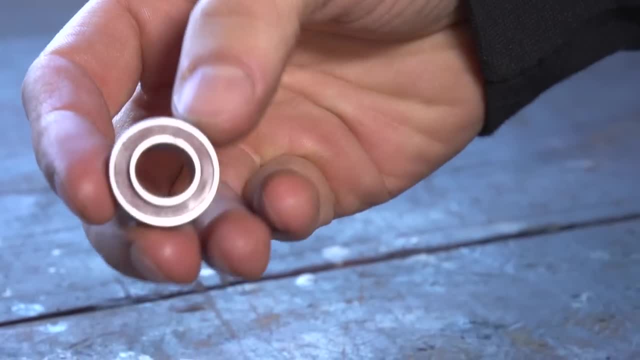 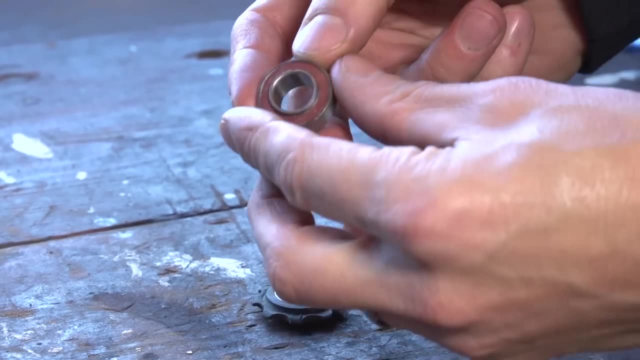 and then you've got this seal that stops stuff getting into the bearings. So they are much more resilient to water and grime than open bearings, but they still need a bit of love occasionally. To do that, you're gonna wanna really carefully just peel that seal off. that's covering the bearings. 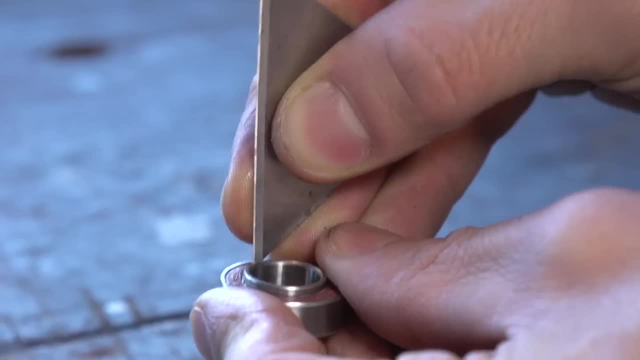 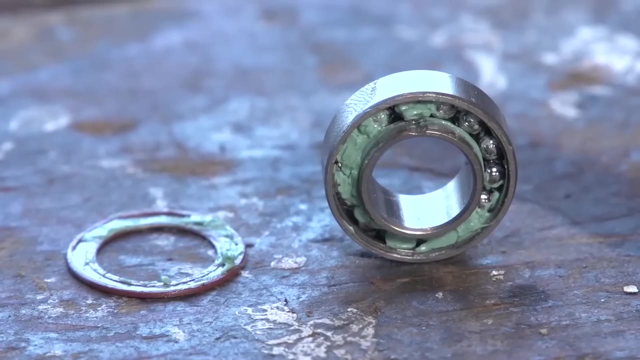 So I'm using a Stanley blade. Obviously, be super careful if you're doing this. You just wanna try and get that seal off without damaging it at all. You can see, I'm just starting to pick it out And you can see behind there. 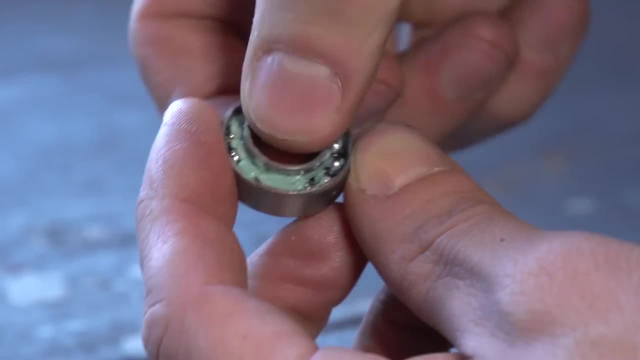 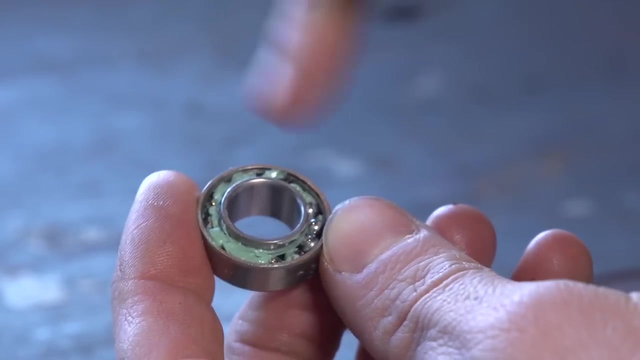 it's nicely greased up, this one, but there's the ball bearings, just like you saw on that open bearing earlier, And this is where same sort of thing applies. really, You wanna clean that out? get your degreaser in there. 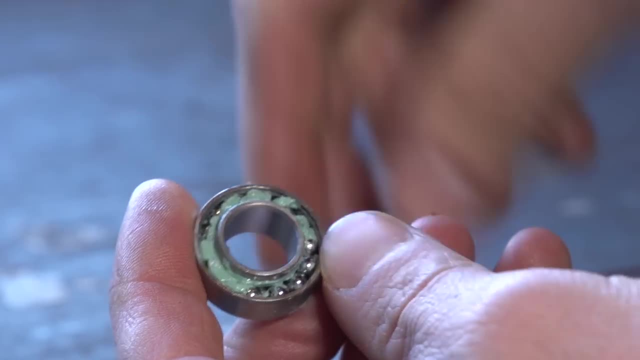 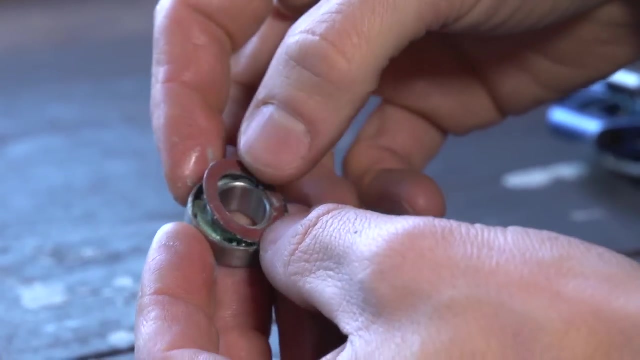 spin that round, get it nice and clear and then re-grease it and away you go. Just be careful to not damage that seal when you're taking it off and also just go around and place it back on nice and carefully. 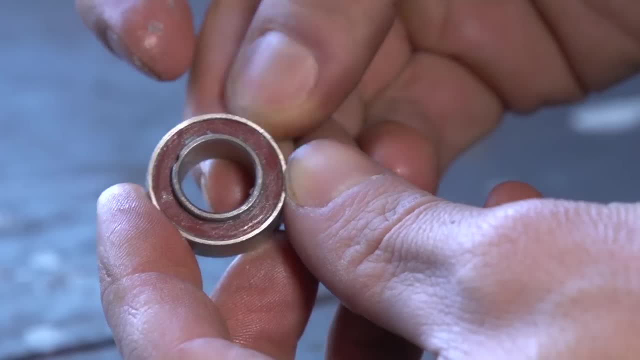 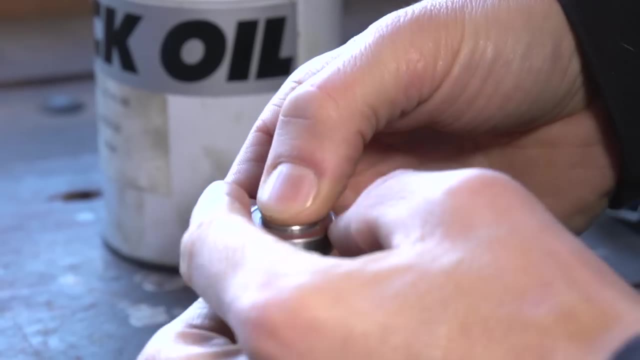 because if that deforms slightly, it can put a bit more friction into that bearing. So once you've cleaned out and re-greased your seal bearing, just give it a little spin in your fingers, see how it feels. If it still feels a bit notchy, you'll have pits in there. 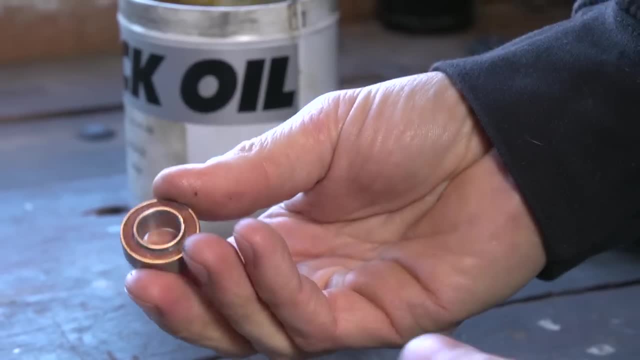 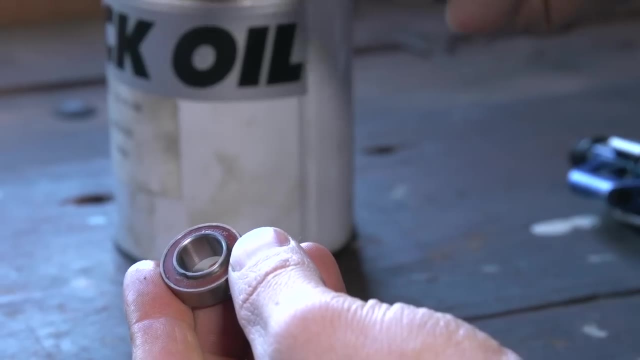 or if it's still a bit loose and not very smooth, then it's time to think about replacing those bearings, And that normally happens if you've just left it too long before you've serviced your bearing With these seal bearings I also like to add 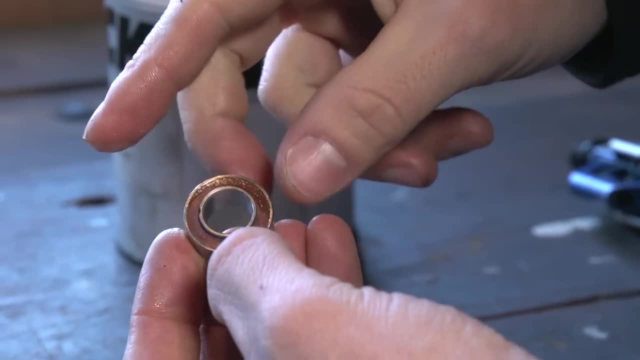 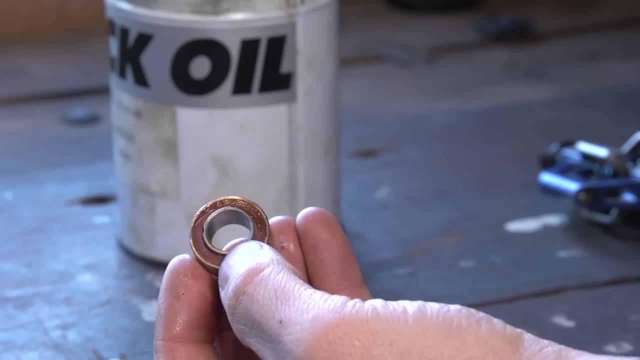 a really nice light coating of grease around the edge of the seal just as an extra barrier to stop any water getting in there. Same goes with a headset, and we've done a video on how to service your headset already, but it's a very similar theory to how we're dealing.